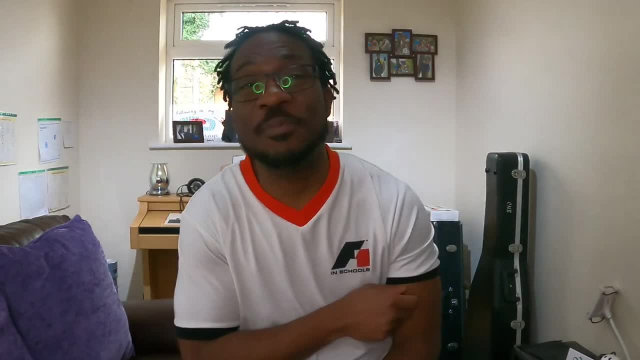 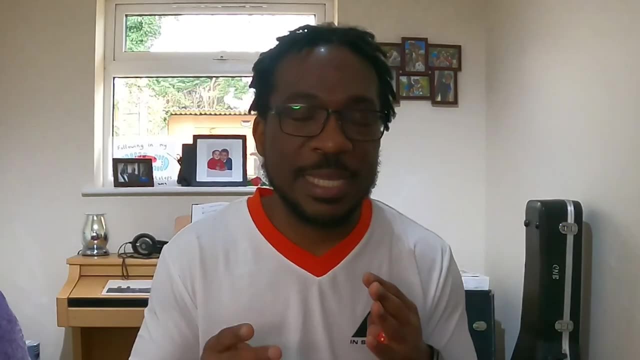 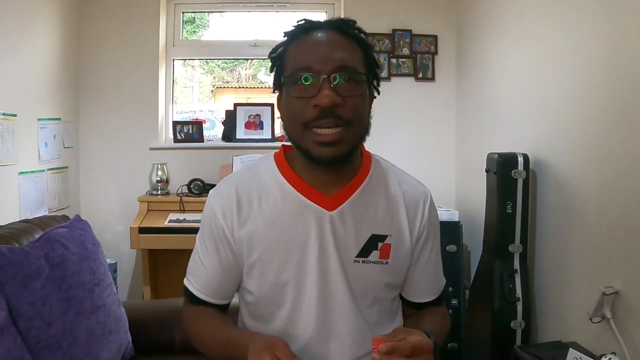 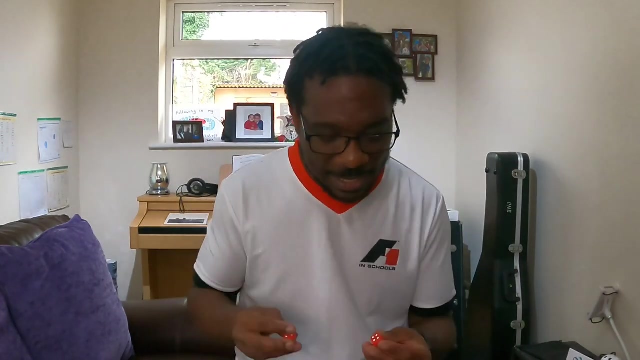 Hello everybody out there, Welcome back to the Rusty Maths channel and welcome back to another of my year 7 series on probability. Now, as we say, year 7, don't forget this is all GCSE spec because we're all training for that, But we're also training to be really good mathematicians. So you know, you can see from the thumbnail it's mainly GCSE, but I call it year 7 because this is stuff I will teach in year 7.. Now I have got my trusty pair of dice there, as you can see. 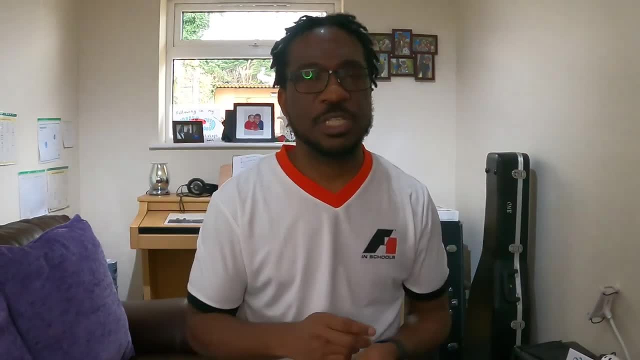 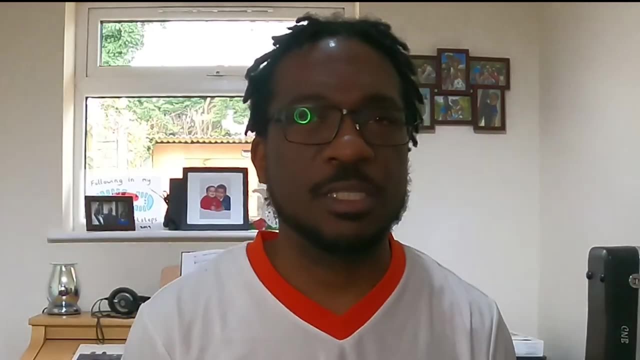 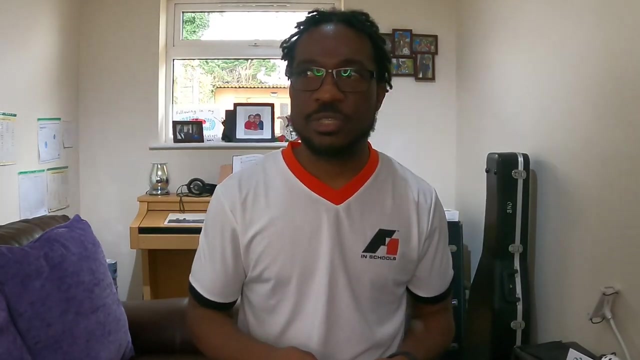 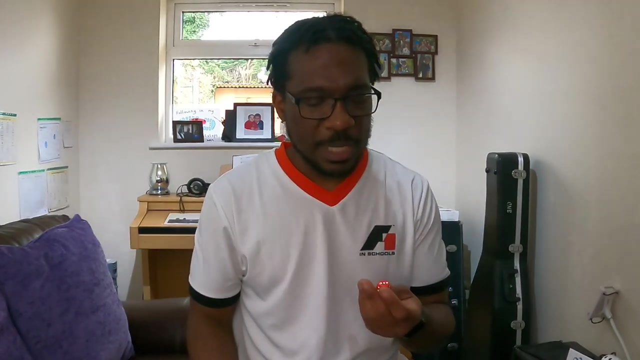 I want to talk a little bit about what we're doing today, which is expected outcomes or expected frequency, and what is this all about? Now, when I get my answer, it's going to be a number, not a fraction or anything like that, mainly a particular number. So what is this all about? So let's start with one of the die. Now let's say I want to throw this die, say 60 times. 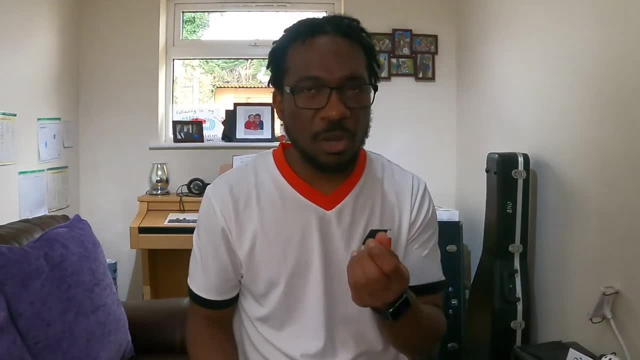 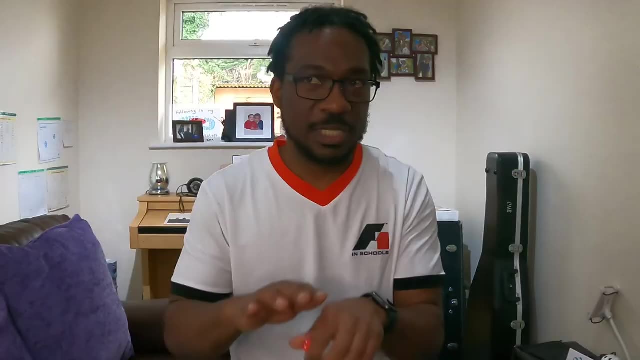 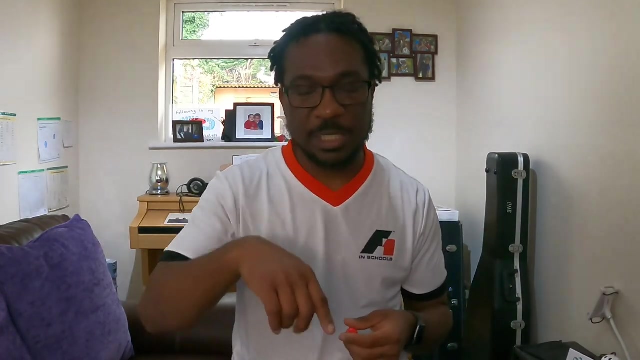 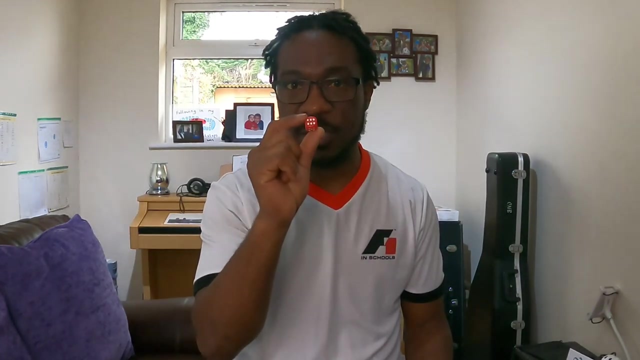 Now, if it's a fair die, then I should see all of these numbers the same amount of times. I should, but I don't, because that's the whole idea of probability. And if you understand what happens with relative frequency and check the link in the description or the pop-out banner popping out there right now, And you can go and have a look at that video, But stick with this and watch it first. And what is this whole thing about? expected outcomes. 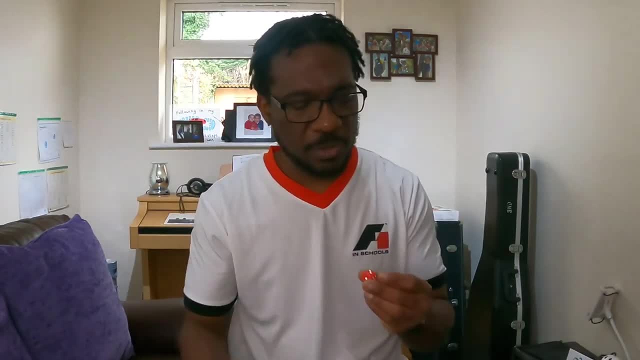 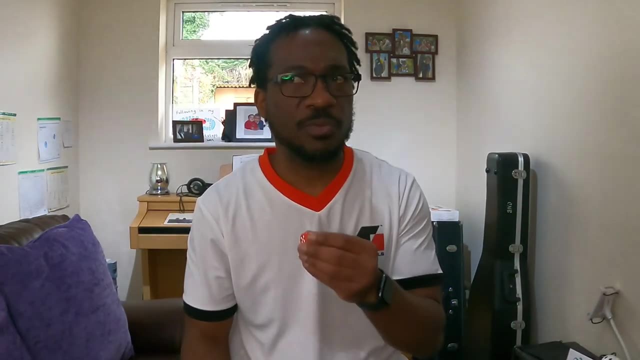 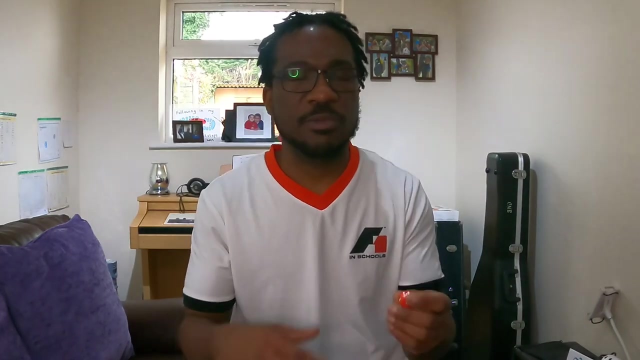 going to be different every time I throw it. So if it's going to be different, then what's the whole point of this then? Well, the whole point is to work out estimates. How can we tell how many times we're expecting to see something? And that comes in quite handy if you're, say, running your 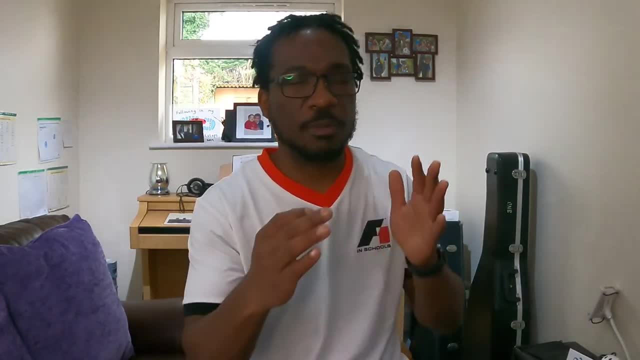 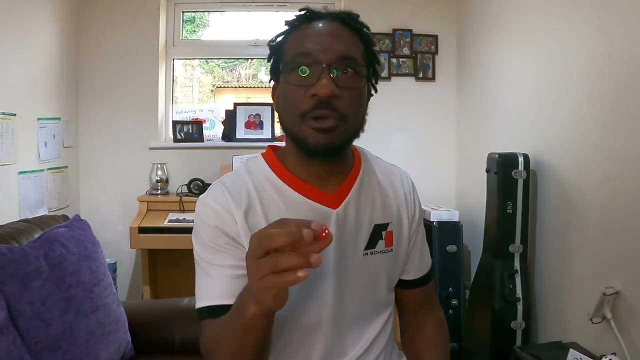 own business and you want to sell a particular product and you know the probability of someone buying that product. What's the expected number of times you expect them to come in that shop and buy that, Or the expected sales value. you're going to make. It all comes in really handy and that's. 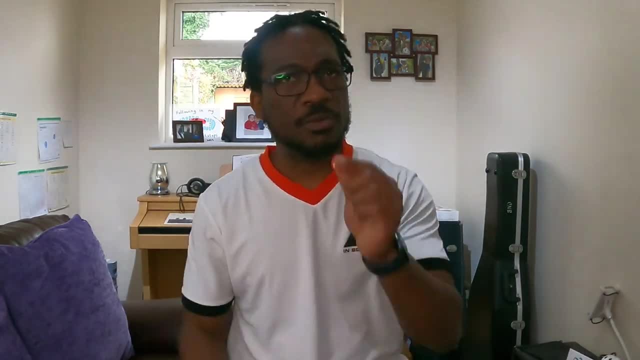 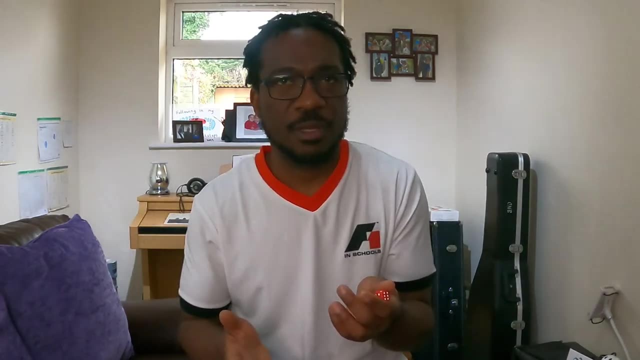 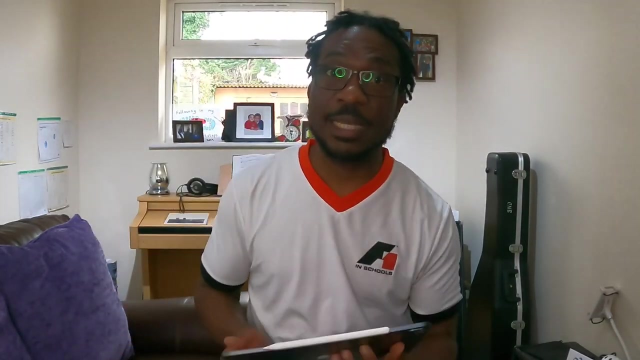 just a silly little example, Anyway. so I'm going to roll my dice 60 times. How many times will I expect to see, say, the number three? And herein comes the whole idea of expected frequency. There's a formula for it. So I'm going to grab my iPad and you follow me now on there, Okay. so first of all, 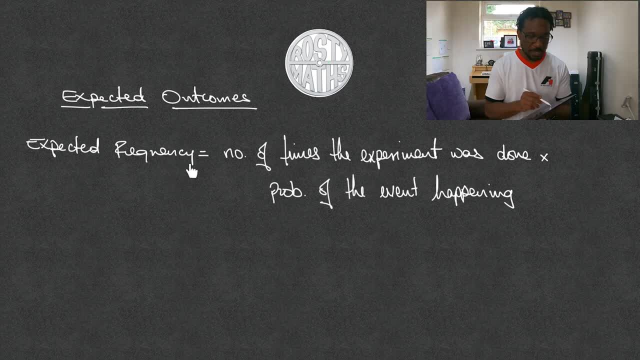 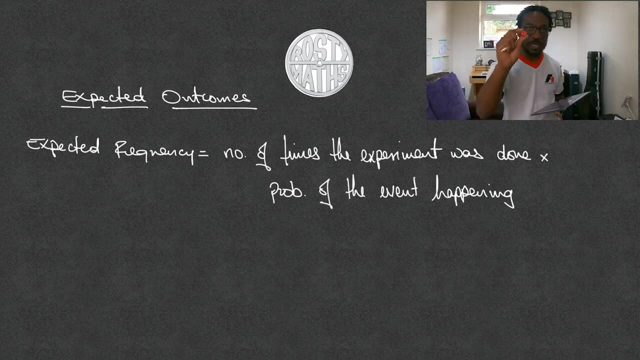 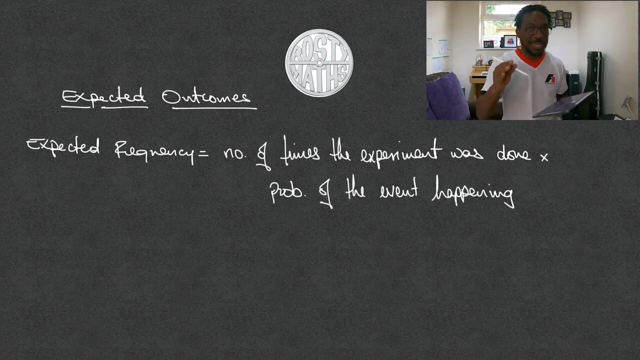 let's see what it is. Let's define it. Expected frequency is equal to the number of times the experiment was done. So, for example, when I was rolling my die, I rolled it 60 times, It was done 60 times, and you multiply that by the probability of that event happening. Now, if this is a fair die, 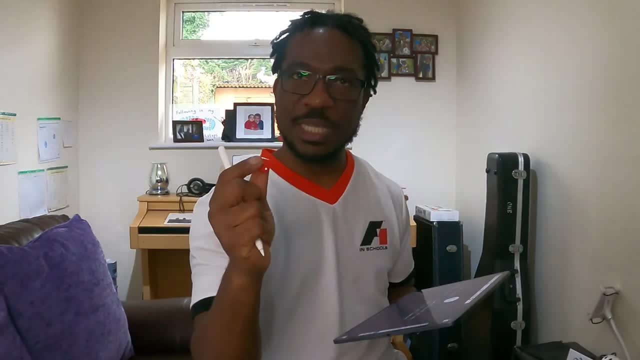 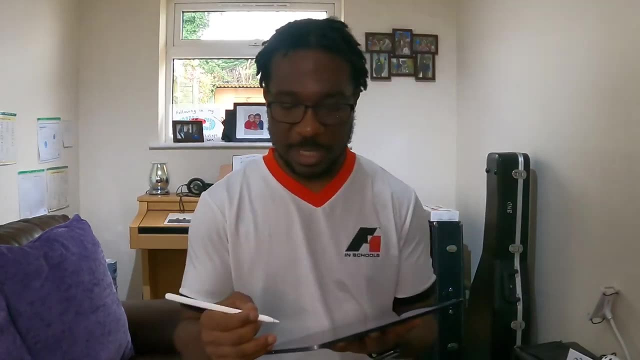 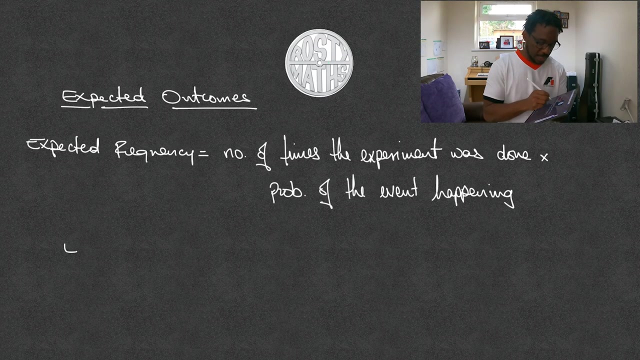 it's not biased. The probability of getting a three is one sixth, because there are six faces on here and there's only one three on here. So now I can say that the amount of times I expect to see a three, So how many times would? 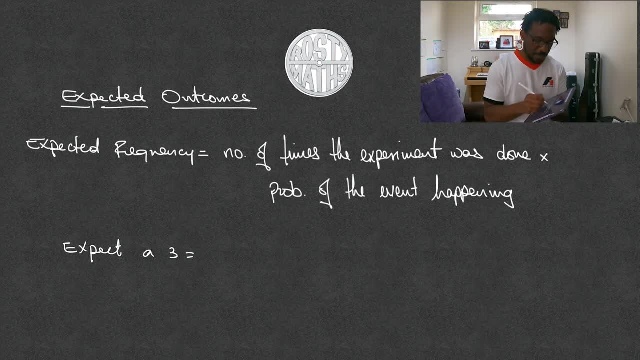 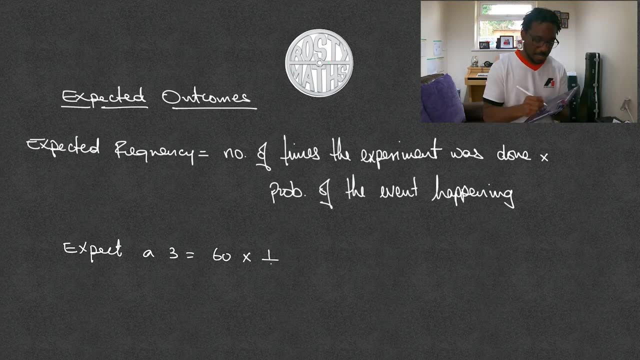 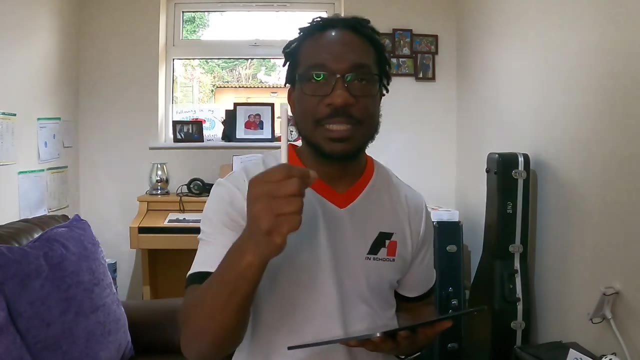 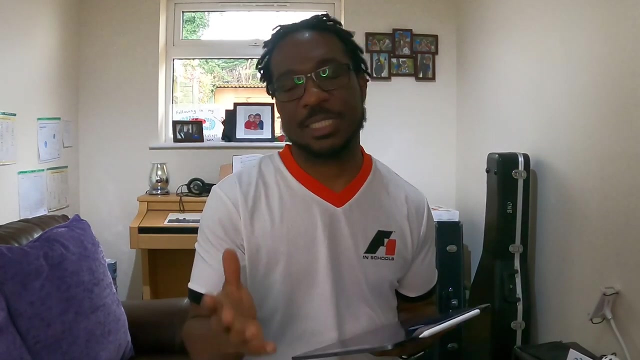 you expect a three. Well, I rolled it 60 times. multiplied by the probability of getting a three is one sixth. So I expect to see a three 10 times. Okay, and that is it to expected frequency. Now, please bear in mind that this is an estimate because, as I said at the top of the video, 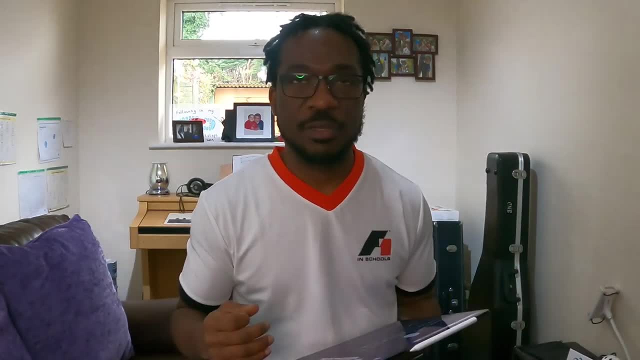 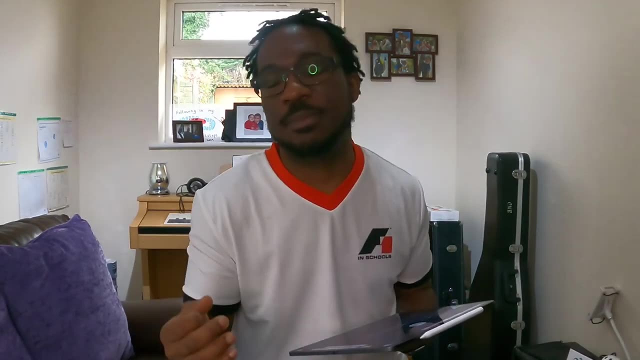 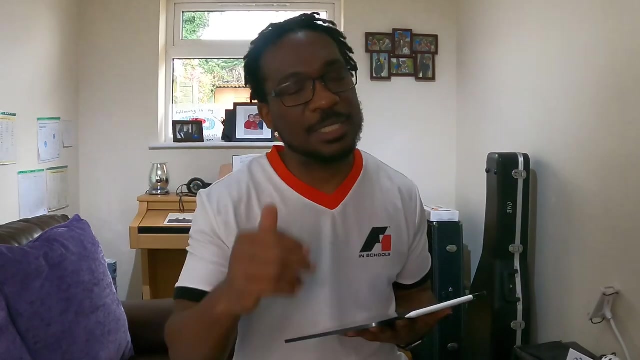 these things will be different every time. And also, even in a perfect scenario, you're not going to get three- 10 times and a one 10 times and so on, Even if a robot's dropping the dice, because all sorts of things are acting on that dice and before it hits the ground. 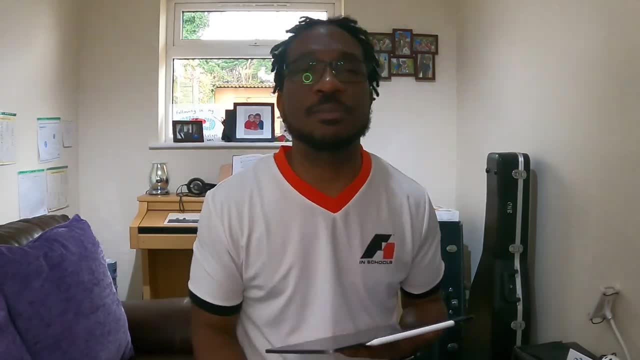 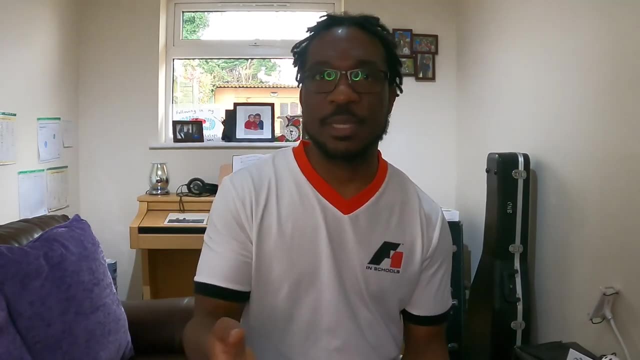 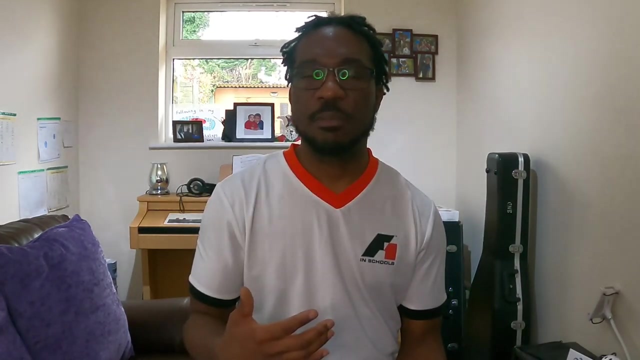 something that you don't expect is going to happen. So that's the number of times I expect to see it. All right, So that brings us to the end of this. I hope you understood that. I hope that you will be able to use this going forward. Now, obviously, this is extendable. You can talk about the number. 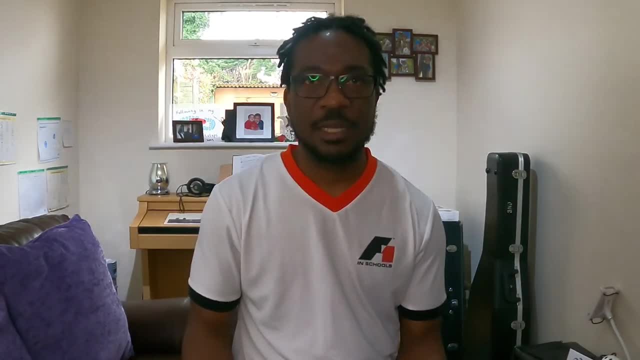 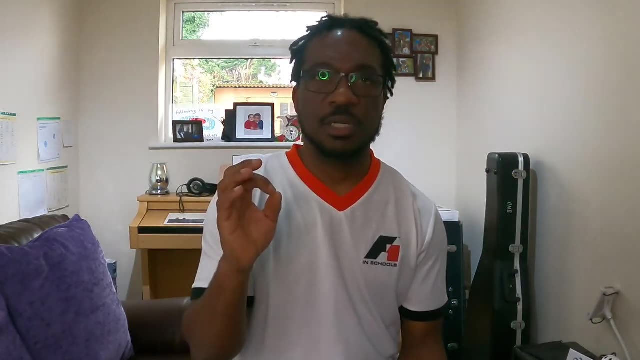 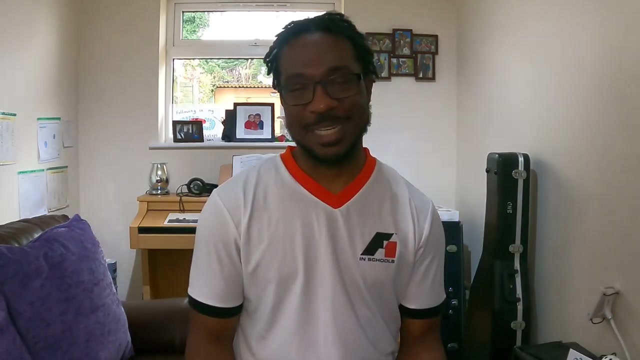 of times you expect to see a number that's bigger than three, say so a four or five and a six, and so on. But that's going to come up in another video when I do the rule for and and or in probability. Anyway, that's the end of it for now, Until I see you in the next video. bye. See you on the next one, Peace. 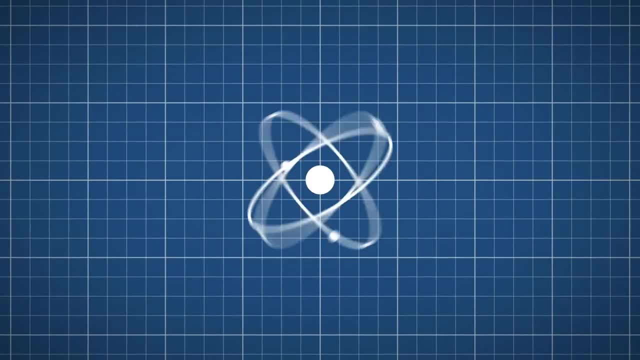 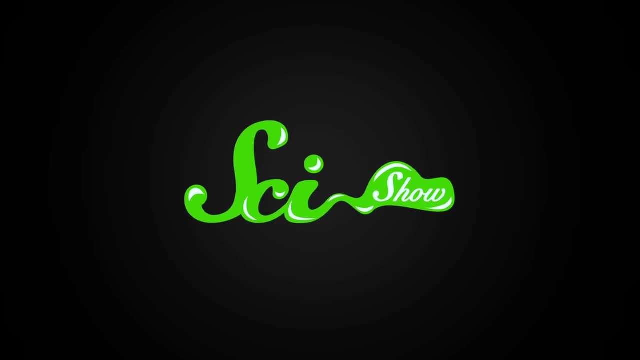 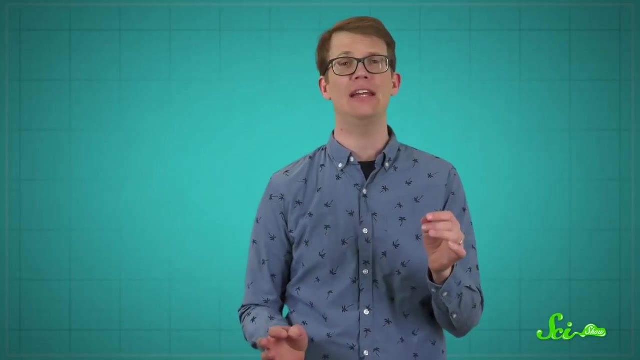 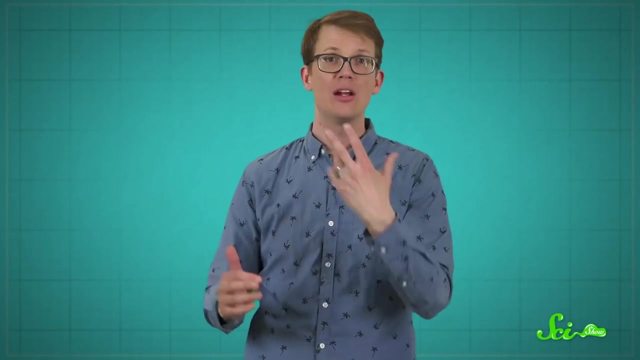 It's not a secret that we haven't been the greatest at taking care of the planet that we live and depend on, but thankfully there are countless conservation efforts happening all over the world to try and undo some of that damage Because, like I guess, better late than never. 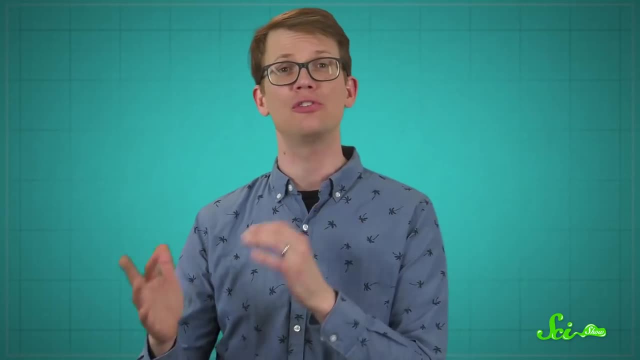 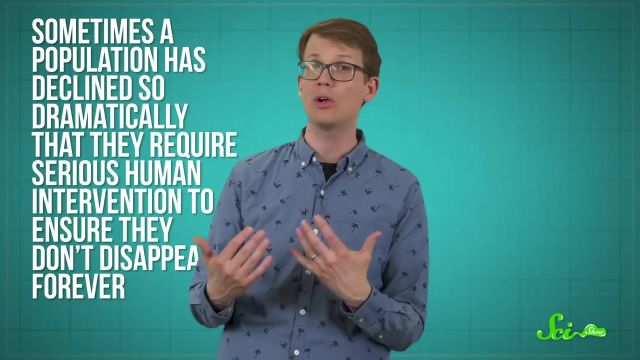 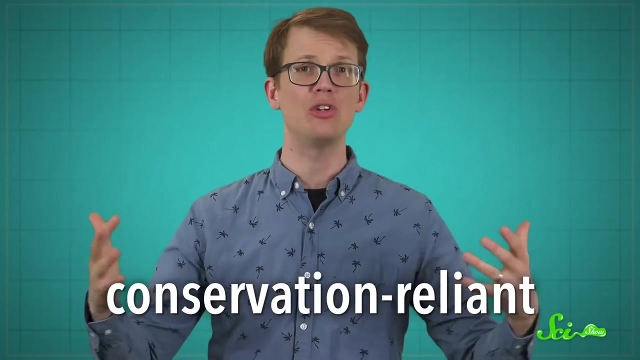 When a species' population is in decline, we can try to find measures to slow and hopefully reverse whatever is going on. But sometimes a population has declined so dramatically that they require serious human intervention to ensure they don't disappear forever. That's when a species can become conservation-reliant. 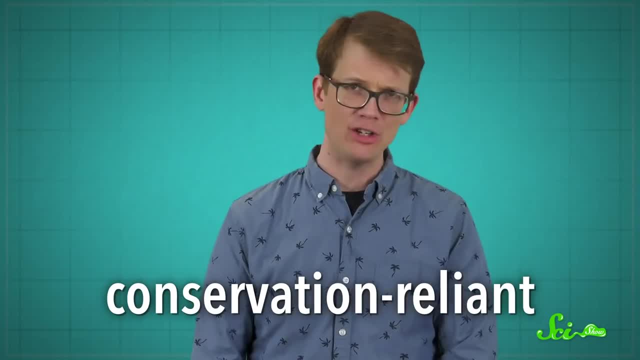 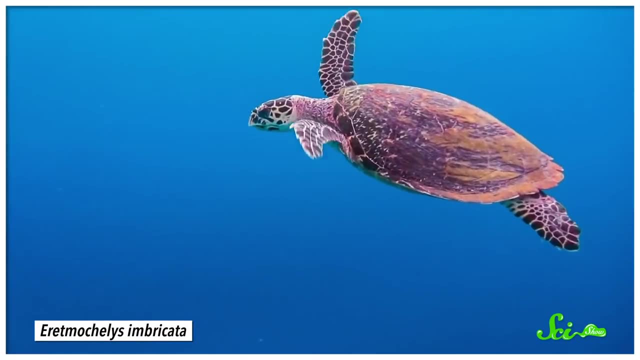 This means that they are in need of consistent, species-specific management in order to survive. What exactly that looks like can vary A lot. Sometimes it means directly protecting a species from whatever is threatening its survival, like invasive predators or a toxin in their 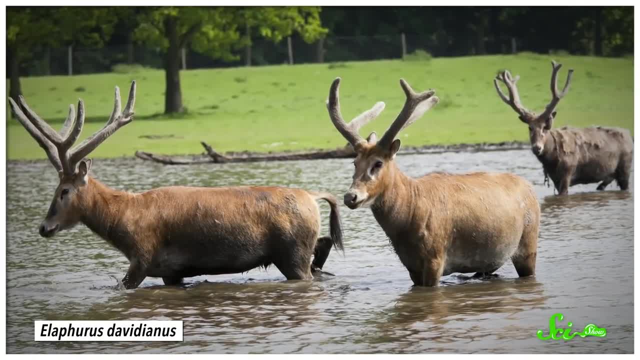 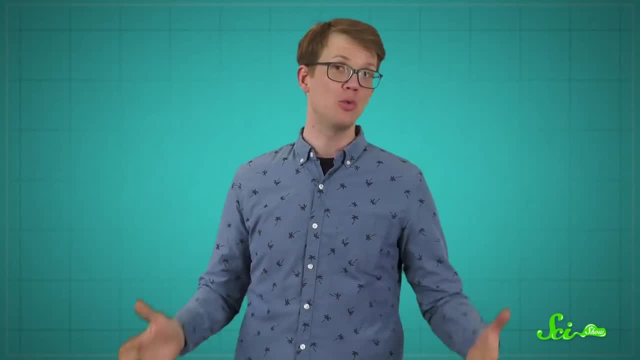 habitat. Other times it means that a species can only survive in human-run breeding programs and may never be able to live in the wild again. The reasons a species becomes conservation-reliant are often our fault, but at least we're stepping up to care for them. 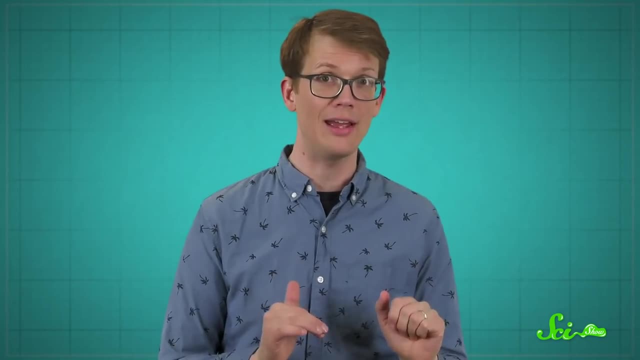 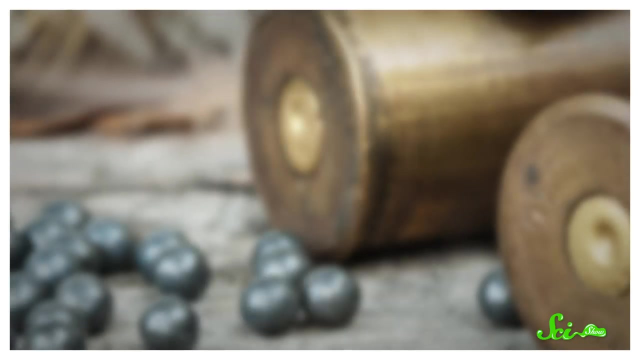 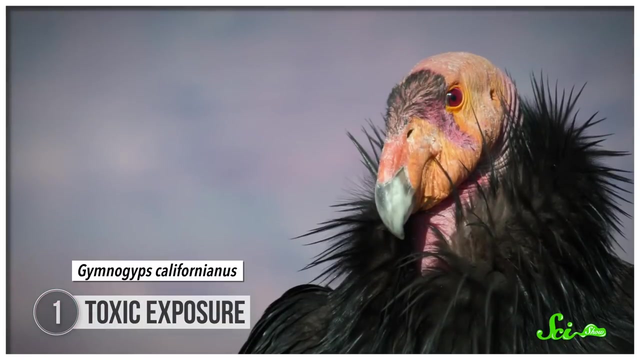 So here are six ways a species can become conservation-reliant and some of the strategies we are using to keep those species alive. Sometimes, when a compound is introduced to the environment, it has a dramatic and often completely unintended effect. Take the story of the California condor. 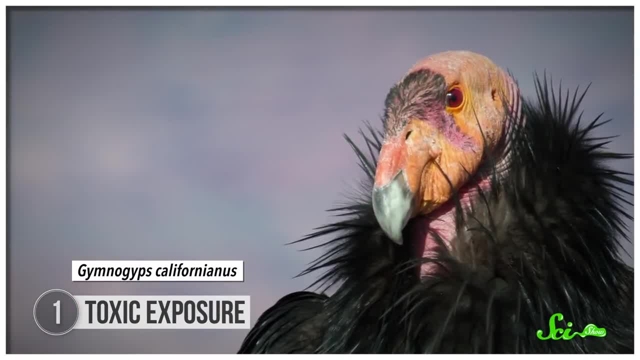 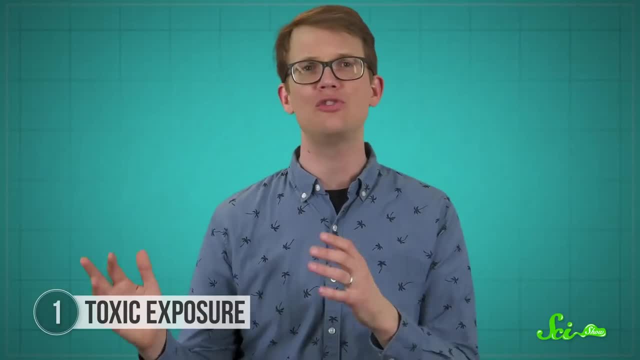 These condors are iconic scavengers and are the largest wild birds in North America, But they've also become severely endangered due to lead poisoning. This happens as condors ingest ammunition fragments in the carcasses they feed on, and it is a major problem. At one time the total condor population was as low as 22 individuals. That's a lot. Thankfully, in the 1980s people did start captive breeding programs to boost those numbers and today all 400 or so living condors are descended from those birds. 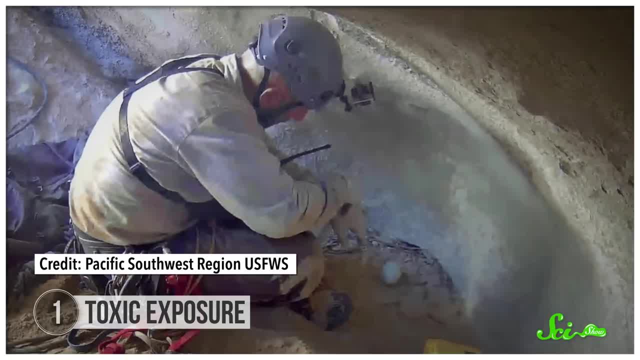 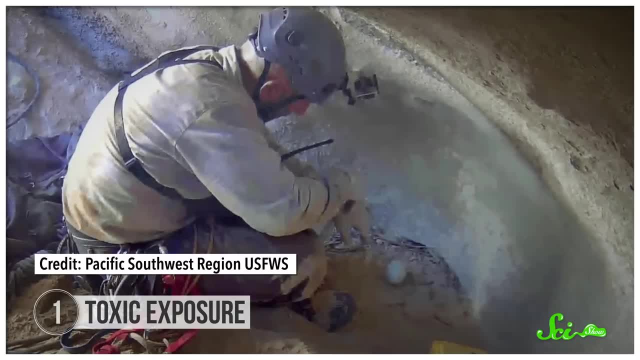 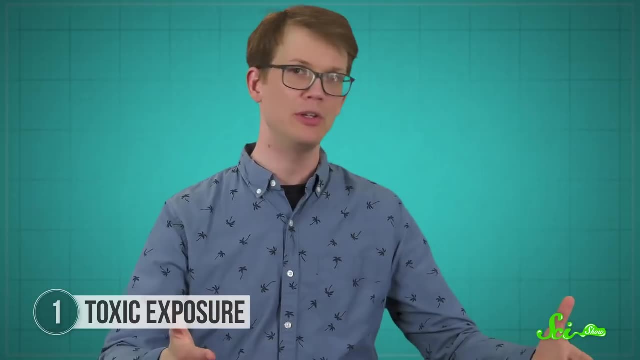 To help with this and keep wild pairs nesting successfully, biologists have put their rock-climbing skills to work, visiting condor nests on cliff faces to swap out any infertile eggs with fertile ones from captive-bred birds. The bigger problem, though, is that these animals are still being poisoned.